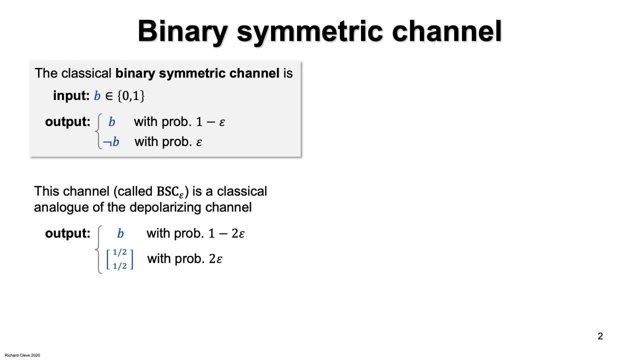 outputs the input bit with probability 1-2 epsilon and the classical maximally mixed state with probability 2 epsilon. The classical maximally mixed state is a uniformly distributed random bit. Now suppose that Alice wants to communicate a bit to Bob and their communication channel is a binary. 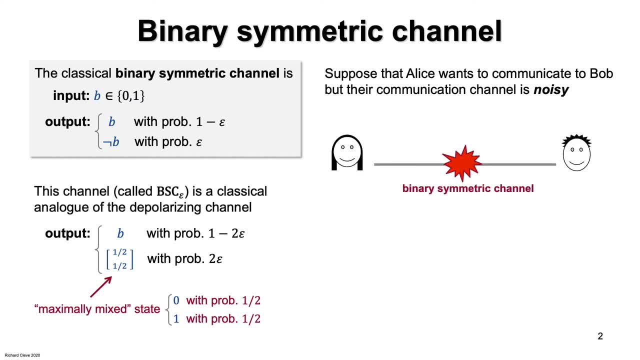 symmetric channel, That is, it flips the bit with probability epsilon. So with probability epsilon Bob receives the wrong bit. So how can Alice and Bob reduce the noise level to a smaller epsilon? The obvious way is for Alice and Bob to get a better communication channel. But Alice, 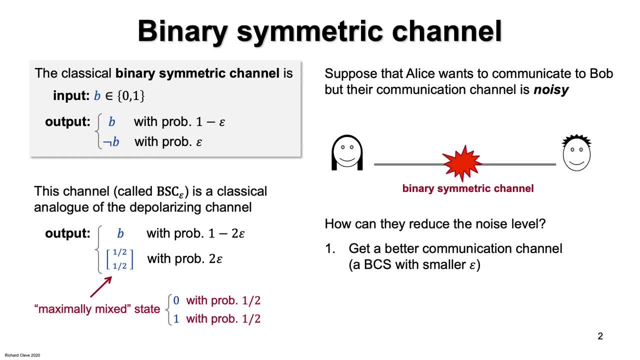 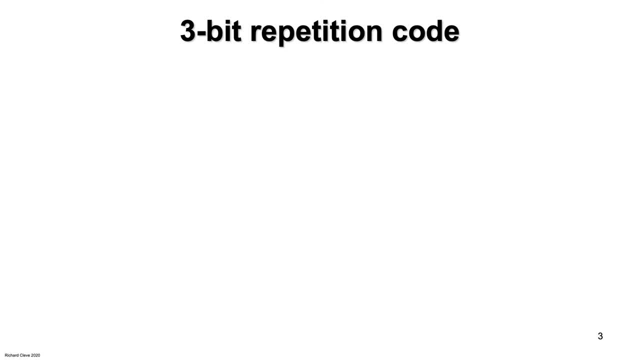 and Bob have an alternative to investing in better hardware, They can use an error-correcting code. Perhaps the simplest error-correcting code is the three-bit repetition code, which works as follows: To transmit a bit B, Alice encodes B into three copies of B. then Alice sends each of these three bits. 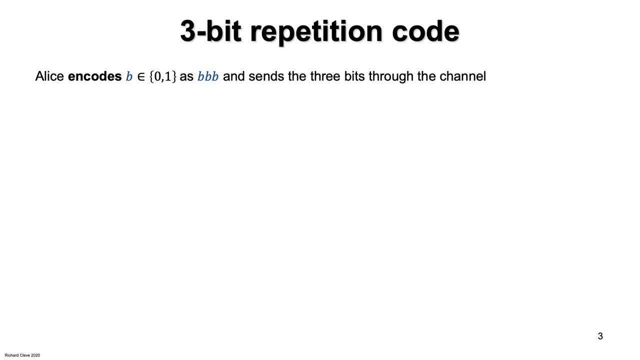 through the channel. Then Bob receives three bits at his end. but the three bits are not necessarily the same. Some of the bits may get flipped by the channel. Bob decodes by taking the original third copy of the NarrowC 1946, taking 6 decodes into one new copy of the NarrowC办. When this is sent to Alice in an error-corrected Naозможно by a leg겠, the console will detect that there is no great mass that is scent-reverting or behavioural. Alicewyeth entries 3 bits in 3 copies of B by 3 copies of B. Then Alice sends each of these 3 bits through the channel. Then Bob receives 3 bits at his end. but the 3 bits are not necessarily the same. Some of the bits may get flipped by the channel. Bob decodes by taking 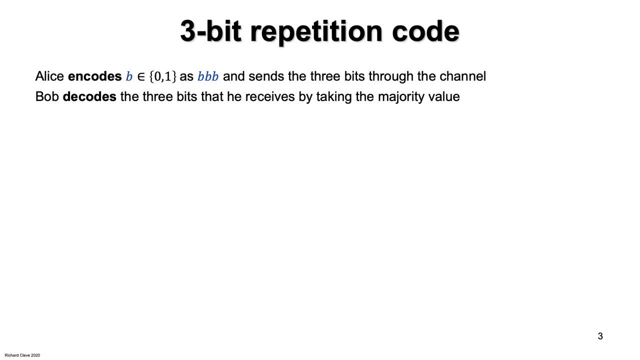 majority value of the three bits that he receives. How well does this perform? The system succeeds if no more than one bit is flipped, because that doesn't change the majority, and it fails if two or more bits are flipped. Assume that the channel 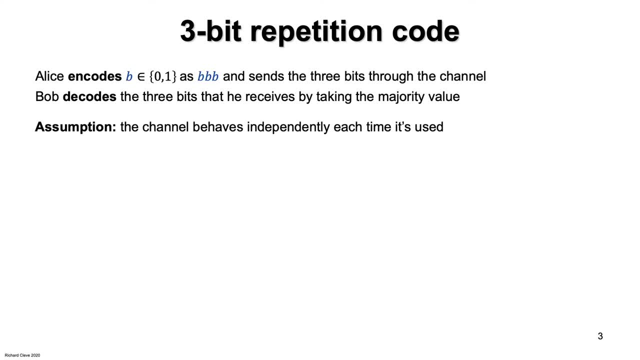 behaves independently for each bit that passes through it, Then the failure probability can be calculated as follows: There are three ways that one bit can be flipped, each occurring with probability epsilon squared, one minus epsilon. and there is one way that all three bits can flip, occurring with probability epsilon cubed. 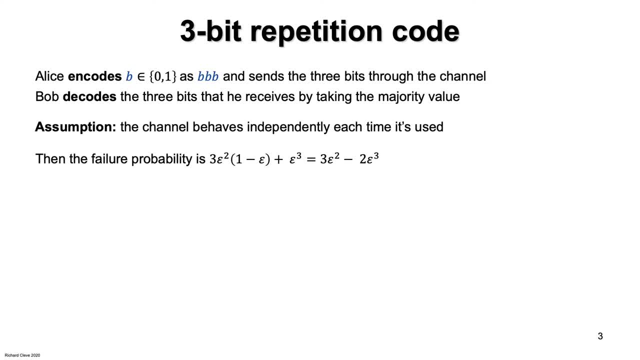 This simplifies through three steps: Three epsilon squared minus two epsilon cubed. Here's a plot of this as a function of epsilon. If epsilon is one half, then there is no improvement. The success probability remains at one half. But this should not be surprising, because if epsilon is one half, 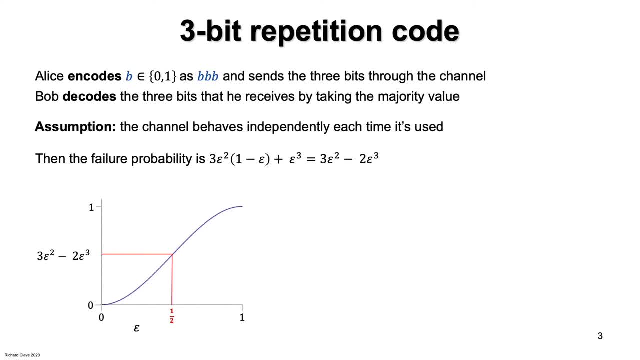 then the channel sends no information, It just outputs a random bit uncorrelated with the input bit. But when epsilon is smaller there is an advantage. For example, when epsilon is one-tenth, then the failure probability from using the code reduces from one-tenth to about one over thirty-five. And if epsilon 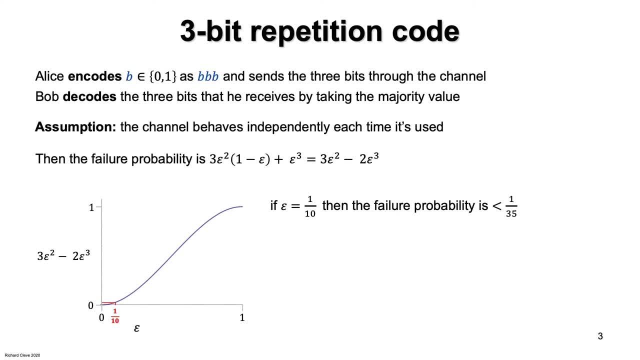 is smaller to begin with, then the reduction becomes more pronounced. For example, if epsilon is 1 over 1000, then the failure probability from using the code is 1 over 300,000, a 300-fold decrease. What price are we paying for this improvement? 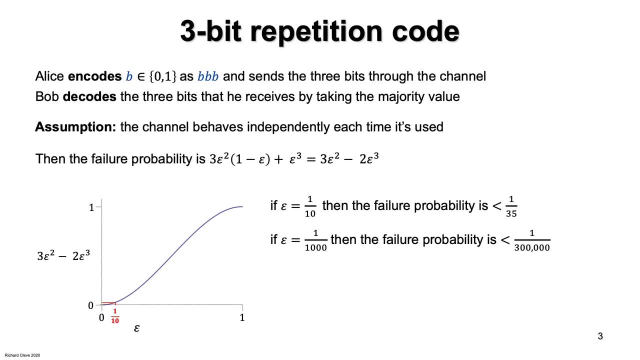 The main cost is that 3 bits have to be sent instead of 1.. The rate of a code is the inverse of the message expansion. The rate of this code is one-third. Each bit of the encoding conveys one-third of a bit of the data to be transmitted. 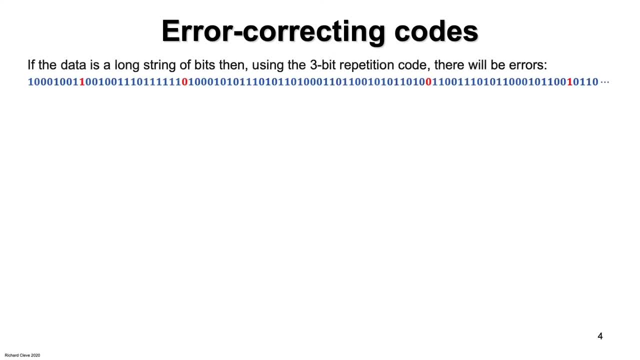 If the data is a long string of bits, then there will be some errors, but fewer errors. using the code. With no code, the fraction of errors is epsilon. With the code, the fraction of errors is 3 epsilon-squared-thousand. 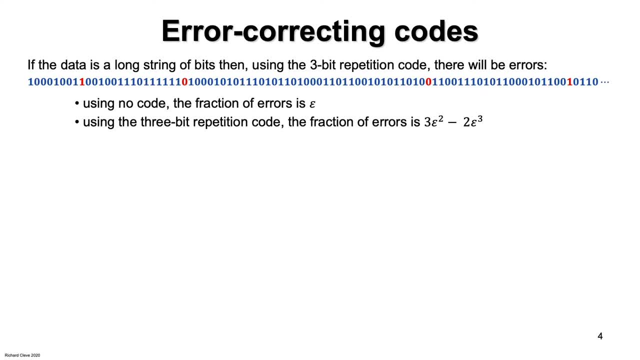 3 epsilon-squared-minus-2 epsilon-cubed. Suppose that Alice wants to send a gigabyte to Bob- That's around 8.5 billion bits- And suppose their communication channel has parameter epsilon as 1 over 100.. Without the code, the fraction of errors will be about 85 million. 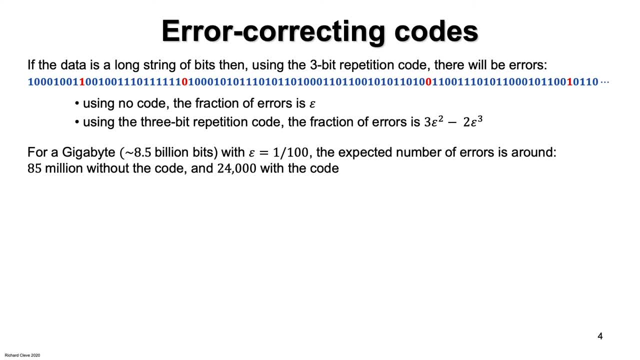 With the code, the fraction of errors will be about 24,000.. That's significantly fewer errors achieved at the cost of sending 3 gigabytes instead of 1.. But suppose that we don't want any errors. Can this be achieved? 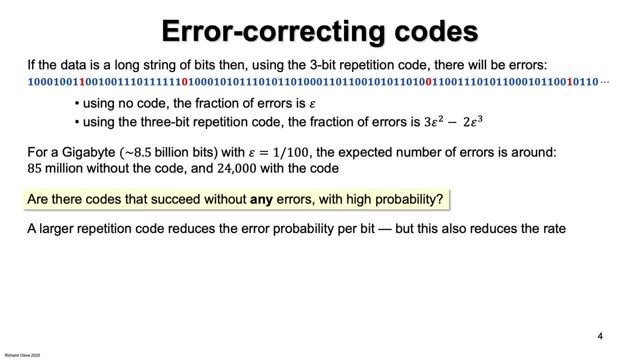 One approach is to use a larger repetition code than 3 bits. That reduces the error probability for each bit, But this also reduces the error probability for each bit. But this also reduces the error probability for each bit. So in this example we can reduce the rate. 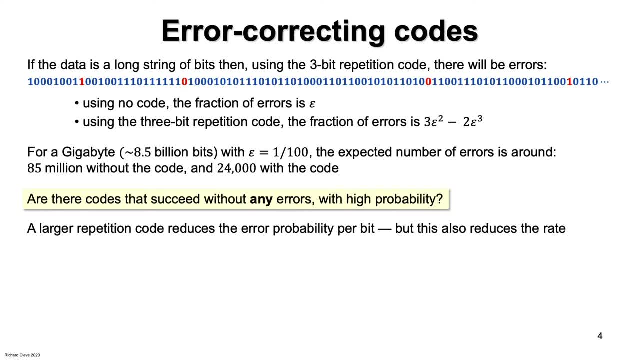 So many more gigabytes would have to be sent. So many more gigabytes would have to be sent. But there are much better error correctan codes than this. But there are much better error correctan codes than this. In fact, there's this amazing result about multibit codes. 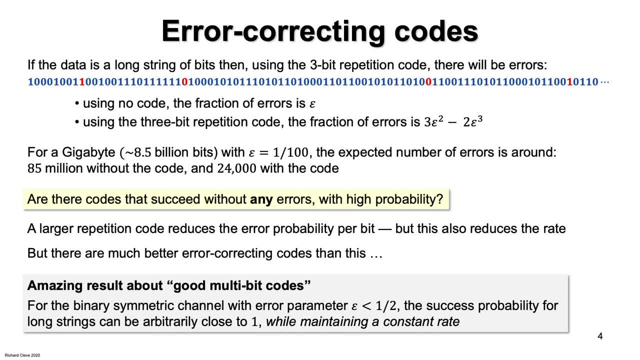 For any binary symmetric channel with any parameter epsilon, that's strictly less than 1 half. The success probability of the whole string can be made arbitrarily close to 1,. The success probability of the whole string can be made arbitrarily close to 1,. 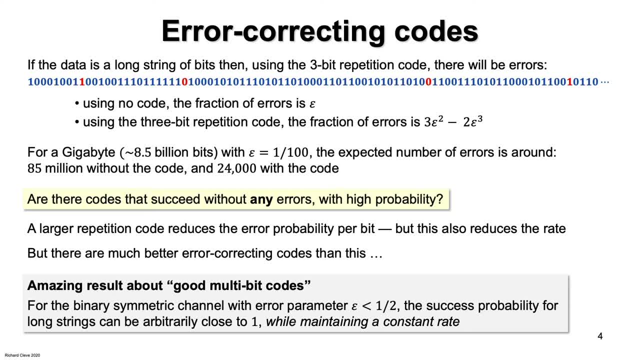 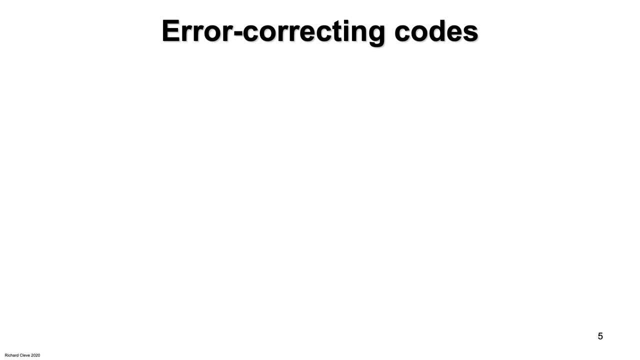 to 1, while maintaining a constant rate. So in fact, Alice doesn't have to send many gigabytes in order to get every single bit through to Bob correctly. To state this result more precisely, let's begin with some basic definitions. Assume 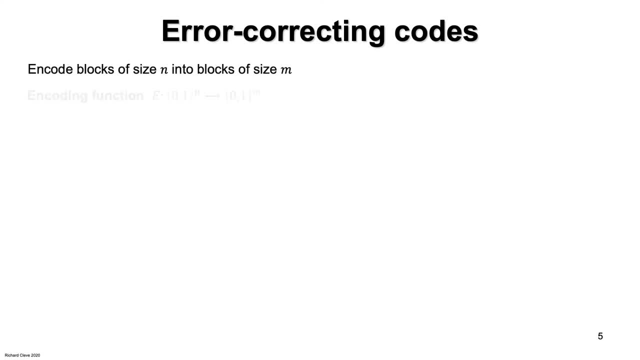 that blocks of m are encoded into blocks of size m and there's a decoding function that goes the other way. Note that the rate of the code is n over m. The smaller the rate, the more bits that have to be sent For any m-bit encoding the channel Bsc epsilon. 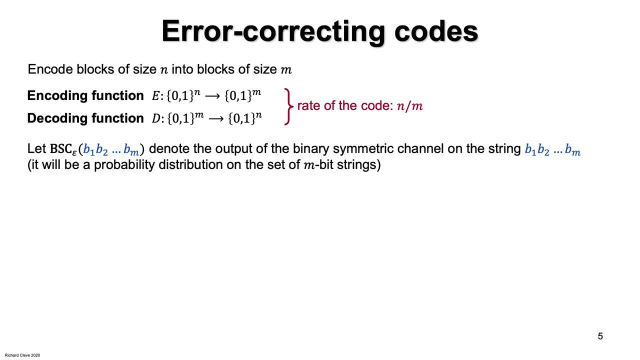 rounds 120 bits of code. All the right bits are encoded into m making. the decoding function randomly flips each of its bits with probability epsilon. To communicate a string, A. Alice applies the encoding function to produce an m-bit string. Then Alice sends those bits through the noisy channel where some of 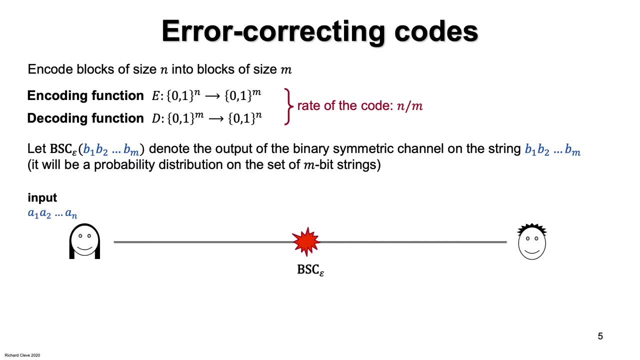 the bits might get flipped. Bob receives the perturbed encoding at his end and decodes it to produce an n-bit string that I'll call A' The error probability is the probability that A and A' differ in at least one bit position. 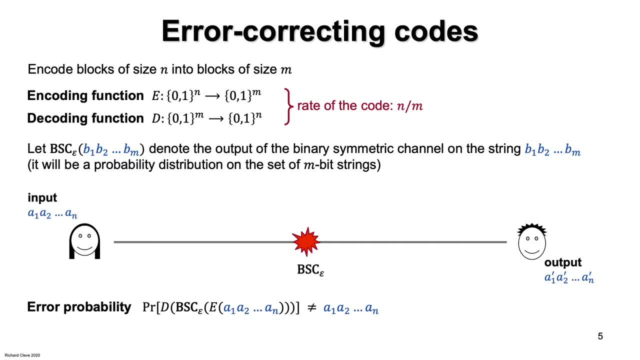 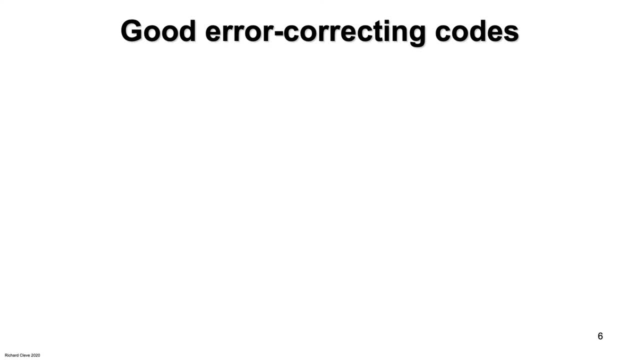 To succeed, every single bit of A has to be recovered by Bob. Next I'm going to state the result about what good error-correcting codes can achieve. Please note that I'm not going to give the details of the construction or the analysis. The theory of error-correcting codes is a. 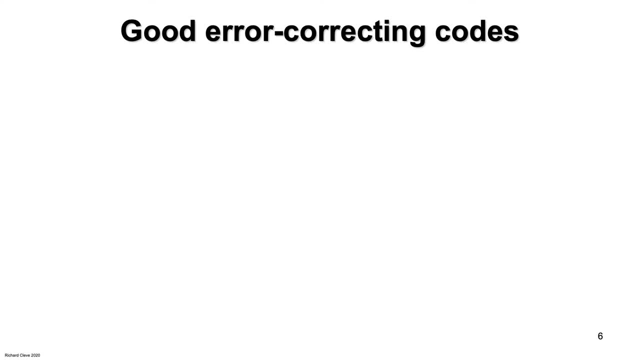 large field of study that could easily take a course of its own. to explain, Suppose that the error model is a binary symmetric channel with parameter epsilon for each bit. What's the best rate possible? The Shannon entropy of the probability vector, epsilon, is defined as this expression: 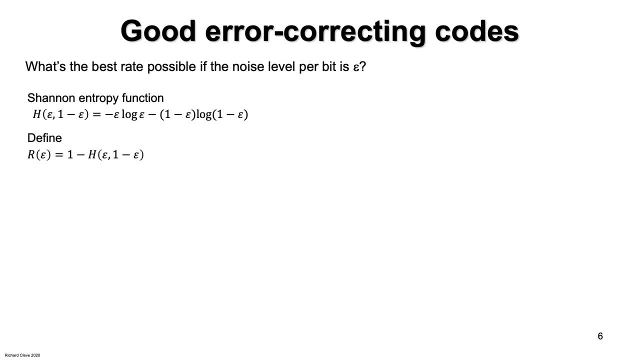 Define R as 1 minus the Shannon entropy. Here is a plot of this function. I'm now going to state the result about good multi-bit error-correcting codes. Let the noise level be any epsilon less than a half. Think of that as a property of the communication channel. that you're stuck. 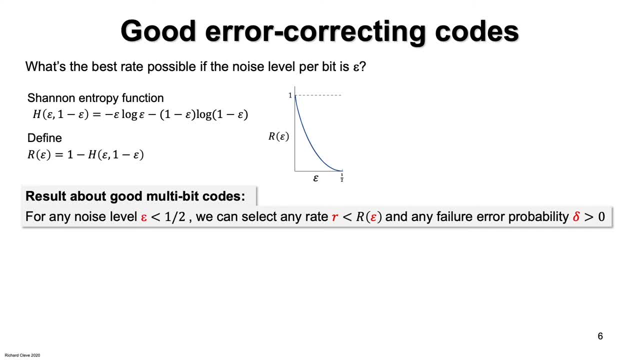 with using. Then you can select any rate, R, as long as it's less than R, of epsilon, As long as it's below the curve, And you can select an arbitrarily small positive number, delta, which is your desired error probability bound. Then there exists an error-correcting code whose rate 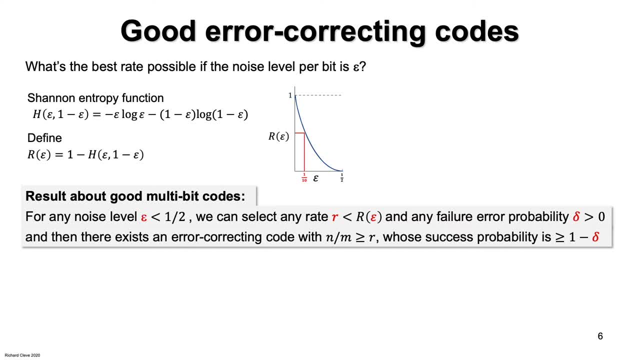 is at least R and whose success probability is at least 1 minus delta. Just to be clear, success means all the bits are successfully transmitted, That there are no errors. There are additional considerations that I'd like to mention, even though I won't go into the details. 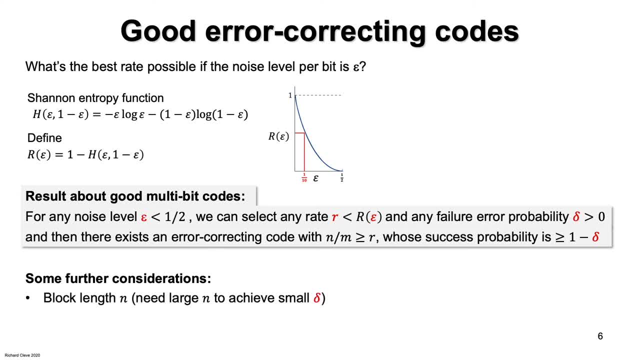 One is the block length: N. The smaller delta is, the larger N has to be. Another is the computational cost of computing E and D. The bottom line is that there are codes for which this can be done efficiently. Okay, so that was a very brief. 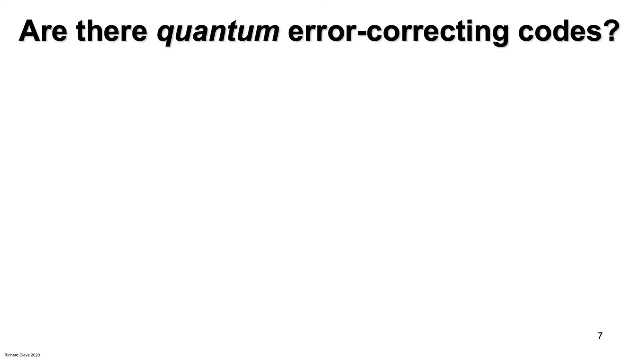 overview of error-correcting codes for classical information. The question is: what happens with quantum error-correcting codes? We started with a simple classical error-correcting code, the 3-bit repetition code. Is there a quantum repetition code? 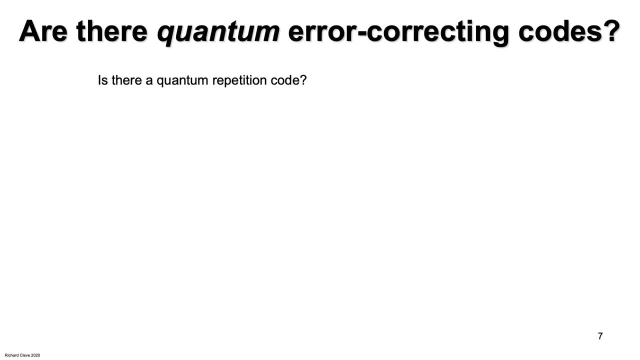 How would that work? Well, we could try encoding a qubit by making three copies of it, And then we could decode by taking the majority value of the three bits received at the other end. How does that sound? Anything wrong with this? 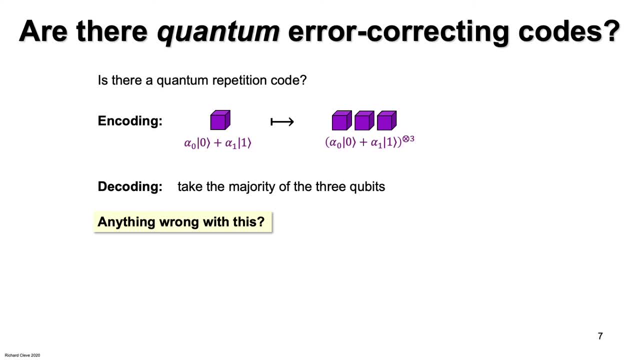 Well, for starters, we cannot make copies of a qubit due to the no-cloning theorem, And it's not even clear how we take the majority of three qubits, So this definitely does not work. It's easy to copy classical information. 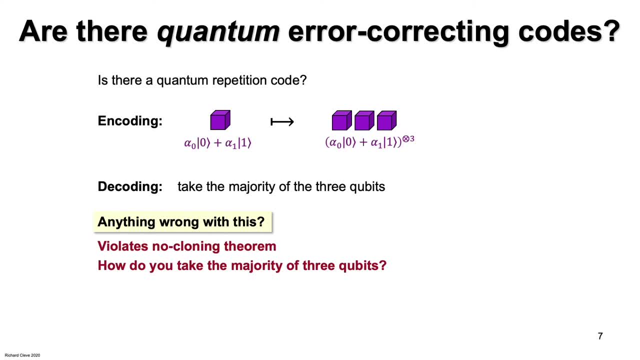 and all error-correcting codes for classical information are based on some sort of redundancy, But the no-cloning theorem kind of suggests that redundancy might not be possible for quantum information. That was the thinking shortly after Shor's algorithms for factoring in discrete log came out. 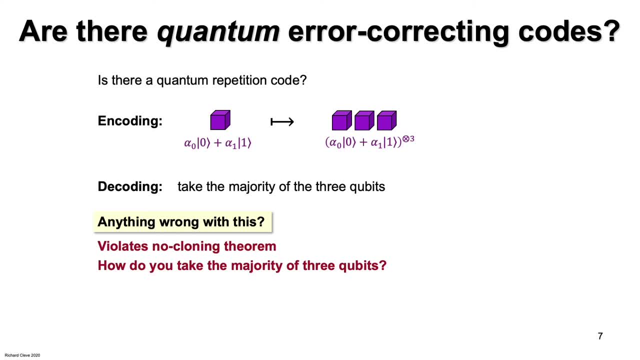 Maybe large-scale quantum computers cannot be built because of the problem of resiliency against noise. Many people thought intuitively that it might be fundamentally impossible to overcome this because of the no-cloning theorem. But this intuition was wrong. In the remainder of this lecture I'm going to show you the first. 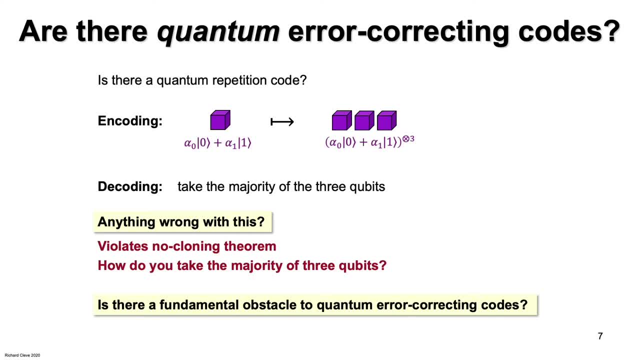 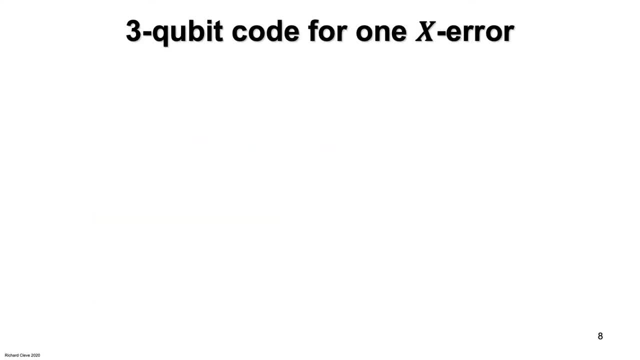 error-correcting code that was discovered by Peter Shor in the mid-1990s. Let's start with a simple three-qubit code that protects against a very restricted error set. Suppose that the only error possible is a poly-X, a bit-flip. 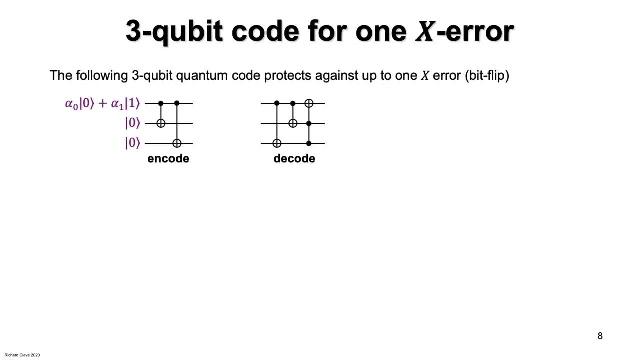 Then these encoding and decoding circuits protect against up to one X error. The encoding circuit takes a qubit as input and produces three qubits as output. Then an error operation that can be one of these four can occur. No error, an X applied. 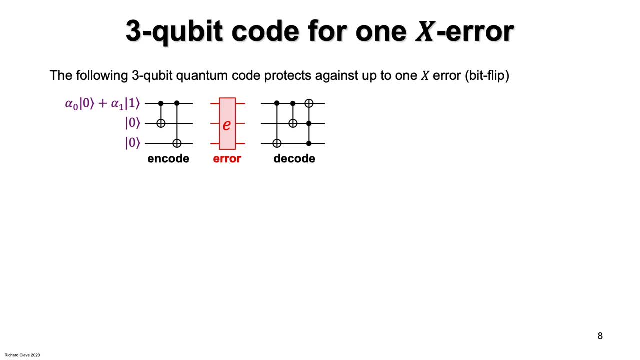 to the first qubit, an X applied to the second qubit or an X applied to the third qubit. Then the three qubits are input to the decoding circuit. It turns out that in all four cases the final state of the first qubit will be the same. 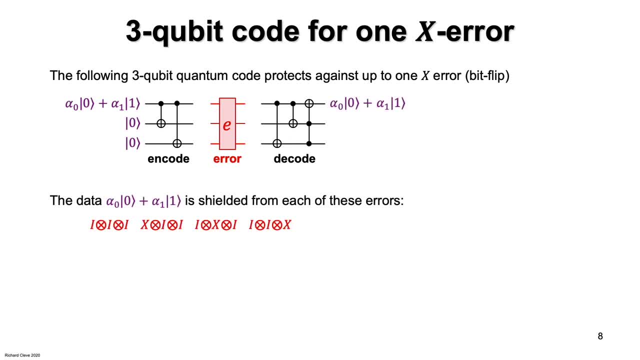 as the initial state of the first qubit. It's a straightforward exercise to verify these, but I recommend that you work through at least some of these cases to convince yourself. If you work out the final states, you will see that the second and third qubits 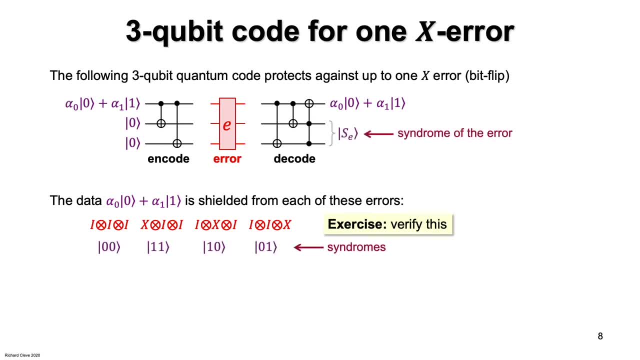 end up with different values depending on what the error operation is. We'll refer to these two qubits as the syndrome of the error. Not only do the encoding and decoding protect the first qubit against the errors, but the decoding process also reveals what the error was. 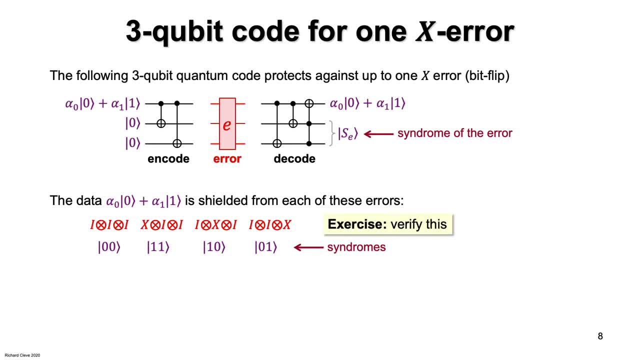 Okay, that's all fine for X errors, but what about other errors? Specifically, what happens if there is a Z error, That is, a Z applied to one of the three qubits in transmission? Please pause if you'd like to think about this. 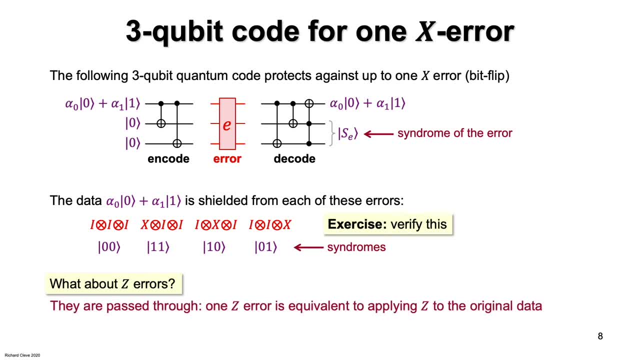 A Z error is not corrected. Instead it's passed through. By this I mean that it's equivalent to applying a Z to the original data, which has the effect of negating the sign of the amplitude alpha 1.. Now here's. 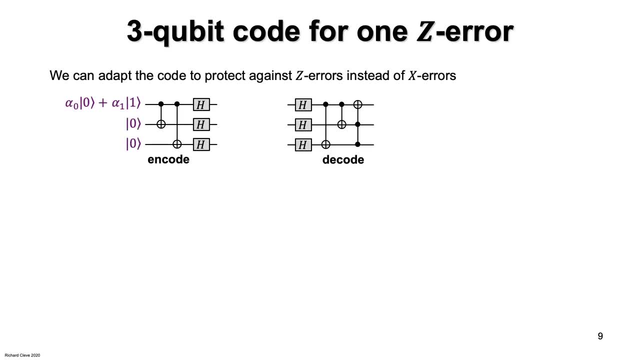 another three qubit code protecting against only Z errors. This code is essentially the same as the previous code for protecting against X errors, but with a layer of Hadamard gates added to the end of the encoding and the beginning of the decoding. What the Hadamards? 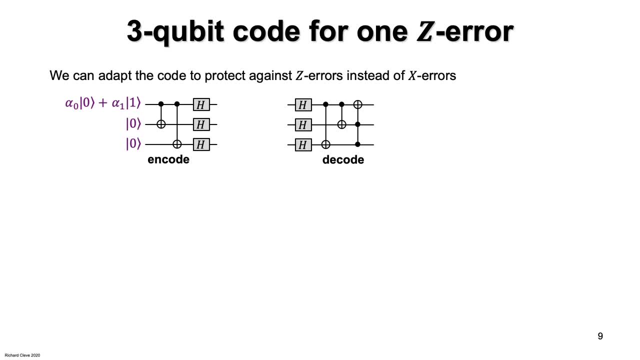 do is convert Z errors into X errors. Think of a Z error and the Hadamard gates. Since HZH equals X, they become X errors and then they are handled as the previous code does. So this is essentially a repurposing of our code for X errors. 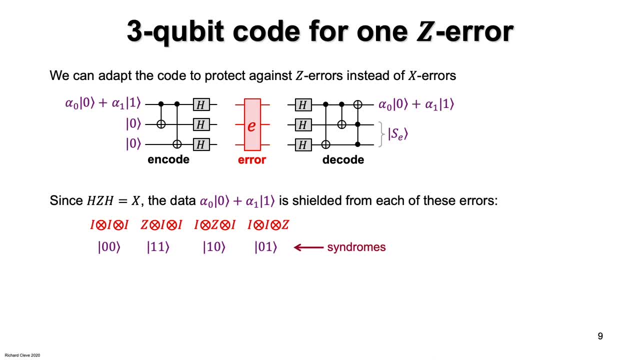 to protect against Z errors instead. Okay, so we can protect against just X errors or against just Z errors. What if we want to protect against any one qubit unitary as an error? This is accomplished by the following nine qubit code: 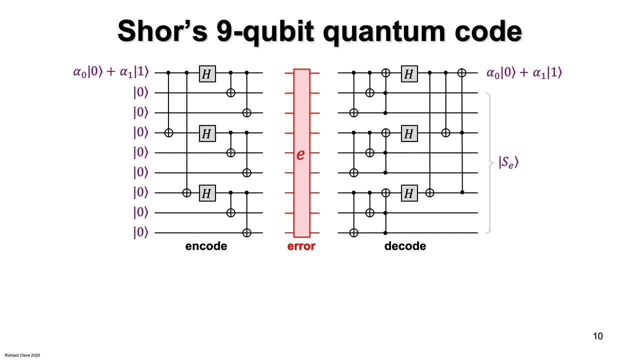 In this code, there is an inner part consisting of three blocks, where each block is a copy of our code for X errors, and there is an outer part which is our code for Z errors. What happens if there is an X error? It is corrected by the inner part. 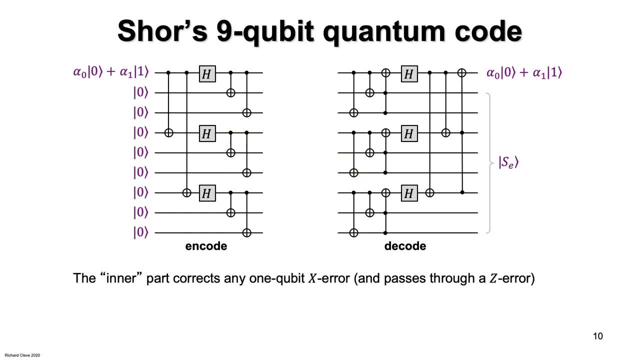 What happens if there is a Z error? A Z error passes through the inner part and then the outer part corrects it. What happens if there is a Y error, Since Y equals IXZ and the phase I makes no difference in this context? 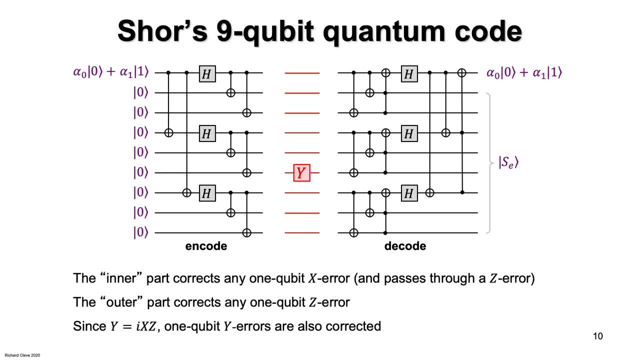 this can be viewed as a Z error and an X error. The inner part corrects the X error and the outer part corrects the Z error. So if there is any poly error in one qubit position, then it is corrected by this code. 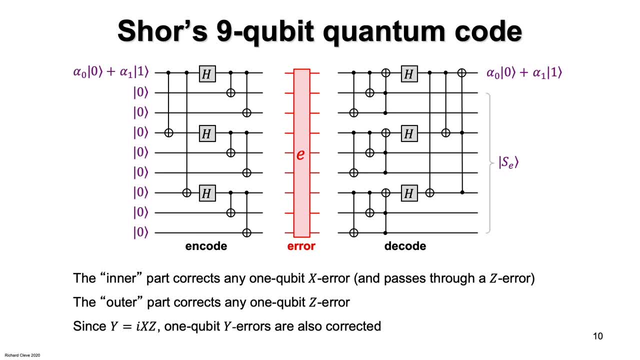 and the final state of the first qubit is preserved. The final state of the eight qubits following the first qubit is called the error syndrome and contains information about which error was corrected. What happens if there is an error in one qubit? 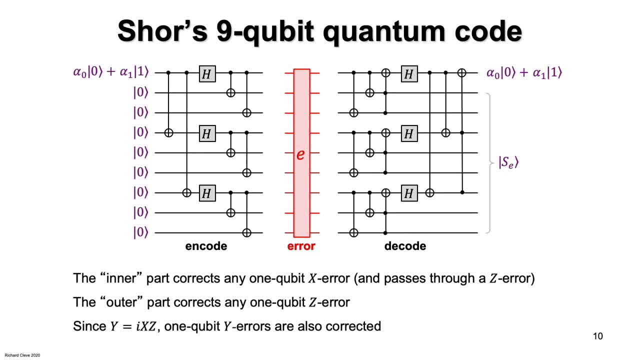 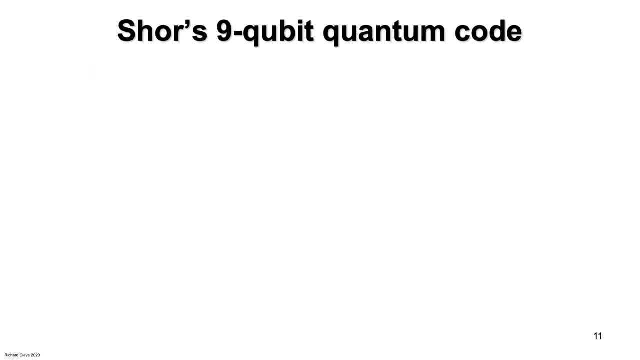 which is a unitary operation other than X, Y or Z. Any one-qubit unitary U is expressible as a linear combination of I and the three polys, and we can work out the final state of this error-correcting code. 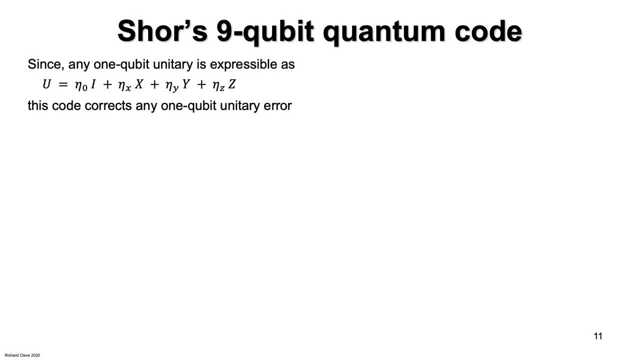 The final qubit ends up in the correct state and the syndrome ends up in a linear combination of the syndromes for I, X, Y and Z. in that position I will leave it to you as an exercise to confirm this. It's an easy exercise. 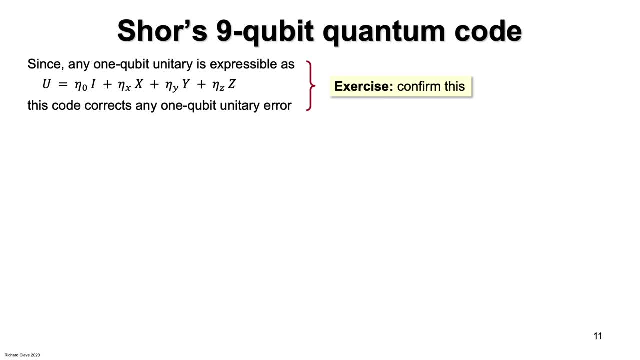 based on the linearity of all the operations. Our discussion of classical error-correcting codes was based on the binary symmetric channel, for which any bit that passes through it flips with probability epsilon. Here's a quantum analog of that channel. A qubit can be flipped in more than one way. 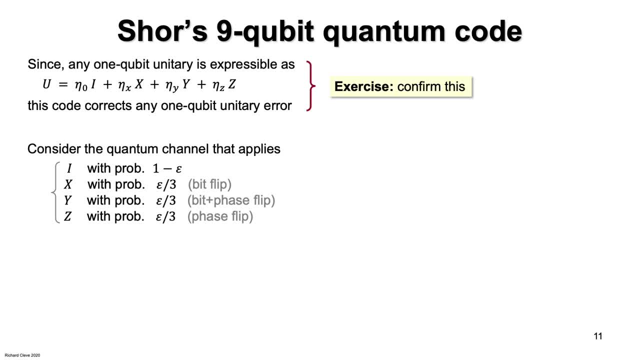 An X error is a bit flip, a Z error is a phase flip and a Y error is like flipping the bit and the phase. This channel leaves the state alone with probability 1 minus epsilon and with probability epsilon does one of the three flips. 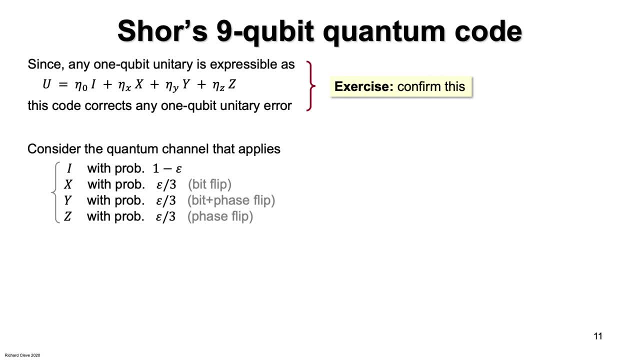 each with equal probability. We've actually seen this channel before, but in a different form. Do you recognize it? This is actually another way of describing the depolarizing channel that maps each state to a convex combination of that state and the maximally mixed state. In other words, it shrinks. 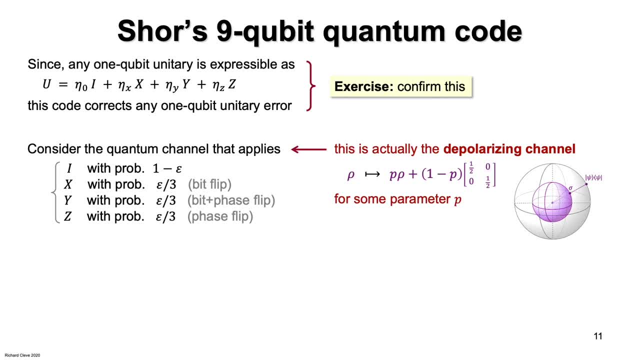 the block sphere towards the center. How do we know that the two channels are the same? I'm leaving this as an exercise to check. It's not entirely trivial and I recommend that you work this out. You might start with any pure state for your qubit. 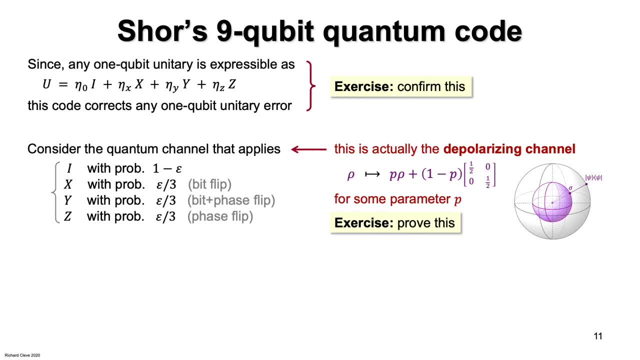 and calculate the density matrix of the state that the channel on the left produces, You'll see that it is equivalent to the channel on the right. What's the value of P as a function of epsilon? Let me give you a hint: P is not equal to 1 minus epsilon. 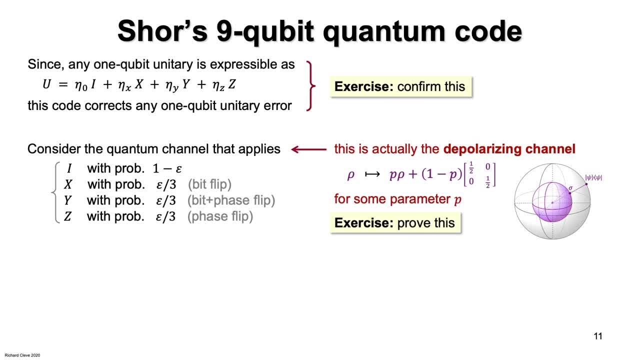 This new way of looking at the depolarizing channel is nice. It's clear that with probability 1 minus epsilon, the state that passes through it is not disturbed, and otherwise the state undergoes some sort of Pauli error. If Atlas wants to communicate. 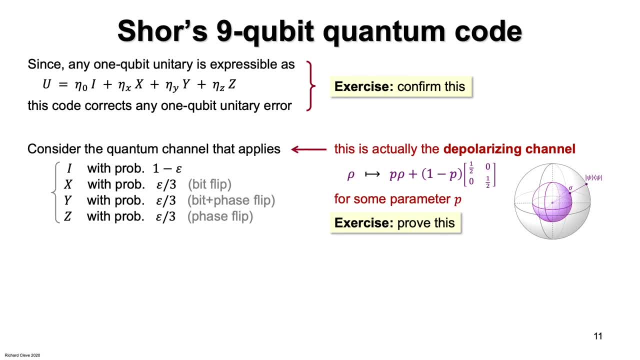 a qubit to Bob through a channel that is depolarizing with parameter epsilon, then if they use the 9-qubit code, the effective error probability becomes a constant times epsilon squared. I don't know the exact multiplicative constant, I haven't worked it out. 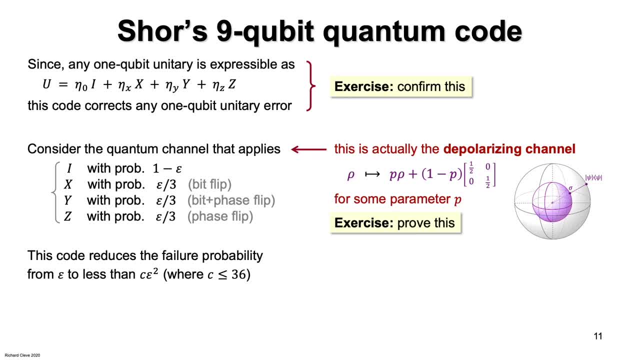 But it's less than 36. So if epsilon is small enough to begin with, then the effect of squaring epsilon is more pronounced than the effect of multiplying epsilon by c, so the effective error is decreased. The cost is that Alice has to send 9 qubits to convey just 1 qubit. 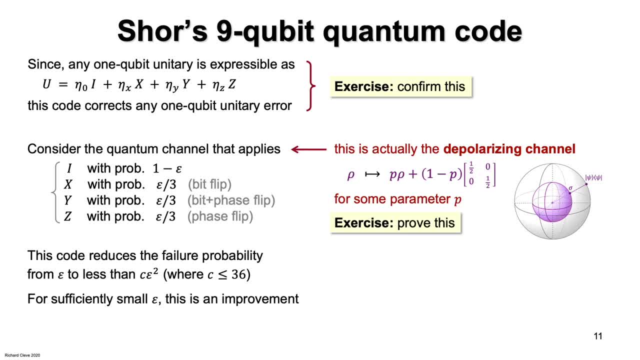 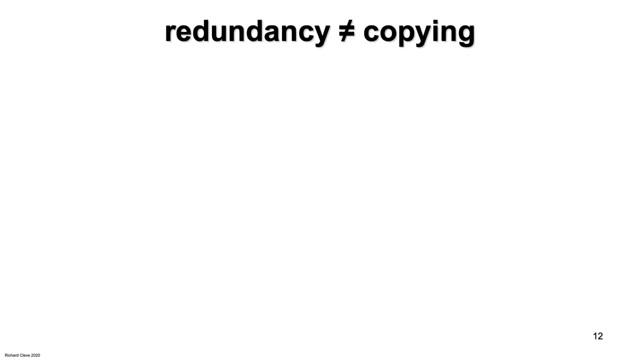 So the rate of this code is 1. ninth, Are there good multi-qubit error correcting codes for quantum information? I will discuss this in the next lecture. Before concluding, I'd like to step back and look at what has been accomplished. Our code encodes a qubit. 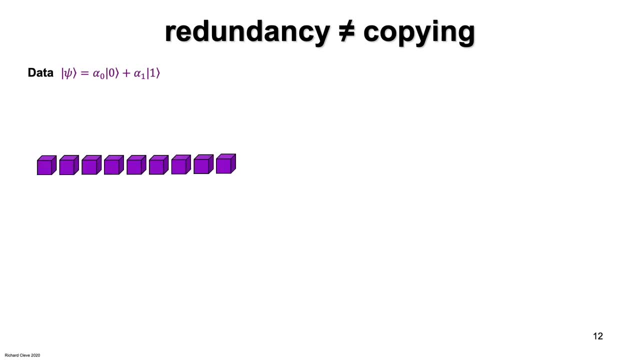 into 9 qubits and this is the state of the encoding. It is a superposition of what's called a logical 0 and a logical 1 state. The encoded state has the property that if any error is inflicted on any one of its qubits, then the data can still be recovered. 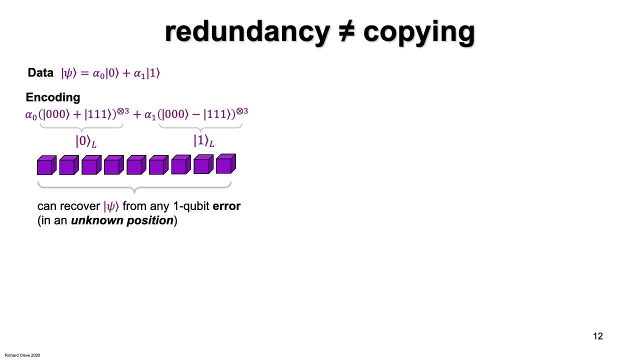 To be clear, note that the recovery procedure is not provided with any information about which qubit has been affected by an error. So which of the 9 qubits contains the data? The answer is that no individual qubit contains any information about the data. This information, 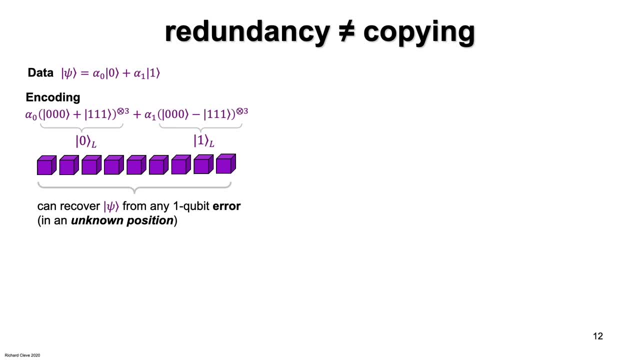 is somehow spread out among the 9 qubits in a manner that makes it robust against a 1 qubit error. There are not multiple copies of the data embedded in the encoding. The natural question is whether there is a more efficient code that requires. 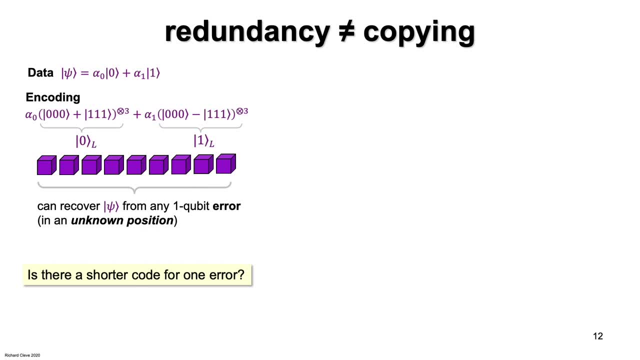 fewer than 9 qubits and protects against any 1 qubit error. This question will be answered in the next lecture. Finally, I'd like to explain a different type of error, called an erasure error. For this type of error, the positions of the affected qubits are known. 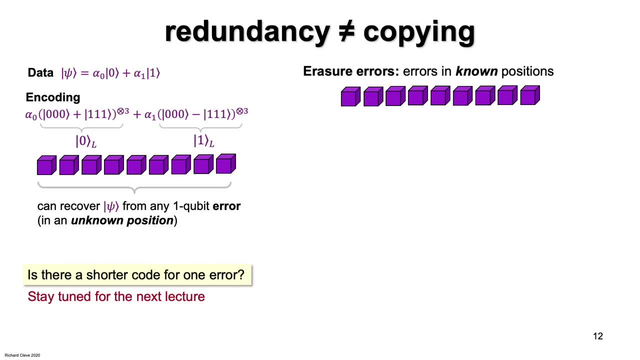 One way of viewing this is that some of the qubits are lost, but we know the positions of the lost qubits and the remaining qubits are undisturbed. For example, suppose that we have our 9 qubit encoding, except we're missing qubits.